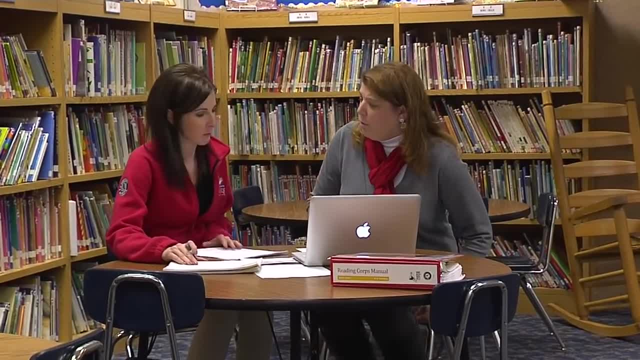 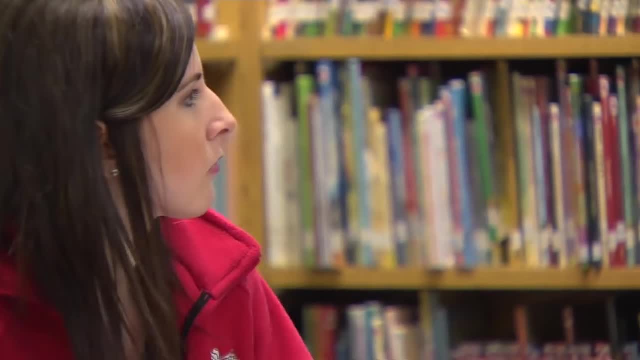 have a few students that I'm kind of concerned about and want to talk about with you. She's the reading specialist here at Middleton and she knows so much and she's so helpful and willing to answer any of my questions any time of the day. She makes herself very available. 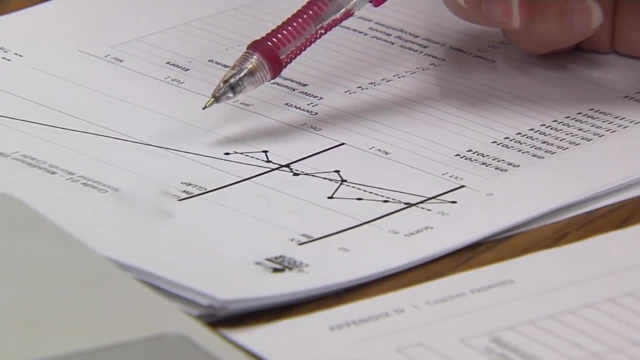 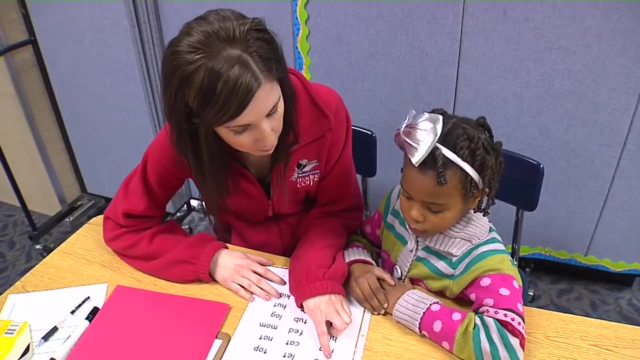 to me And I have been doing this, The at-home reading with her. Okay, And then we'll just sit down once a week to do a data meeting. talk about how every child is doing. that's in the program When I point underneath. 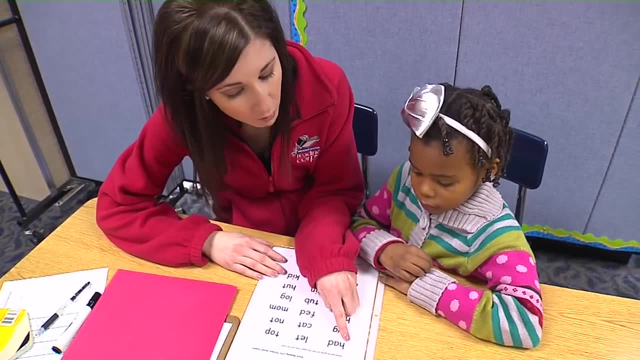 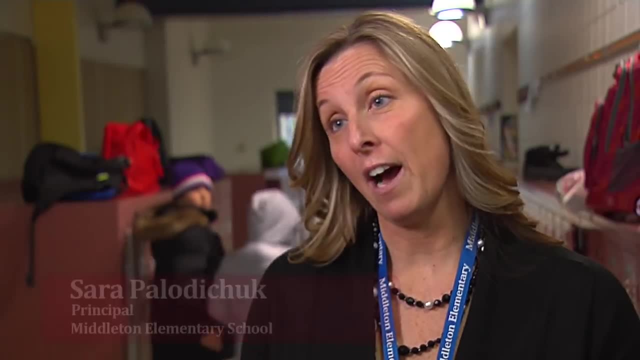 a letter, you say the letter sound okay. It's not just coming in sitting and doing lessons. The lessons are very structured, They're very detailed, They're really about filling those gaps where the students have and then that ongoing progress monitoring. 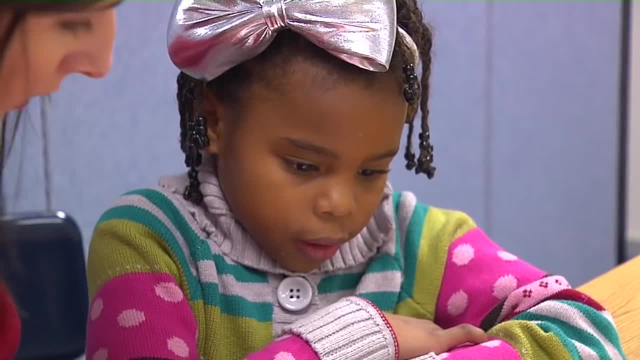 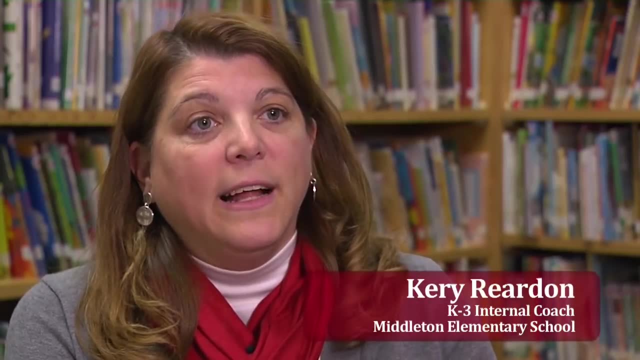 Let Let Okay, Callie would have a student with her in her room and then I will sit in and watch The interaction between Callie and the students. I will look at the intervention, which might be, for example, a duet reading. 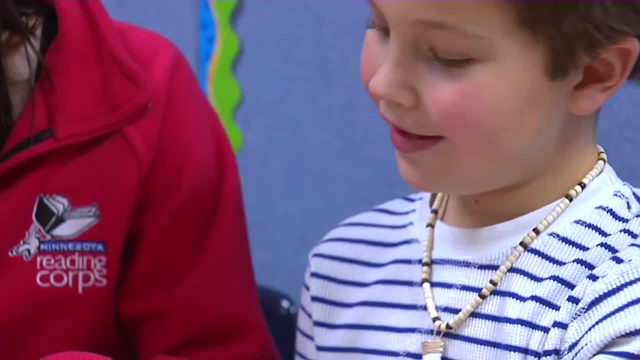 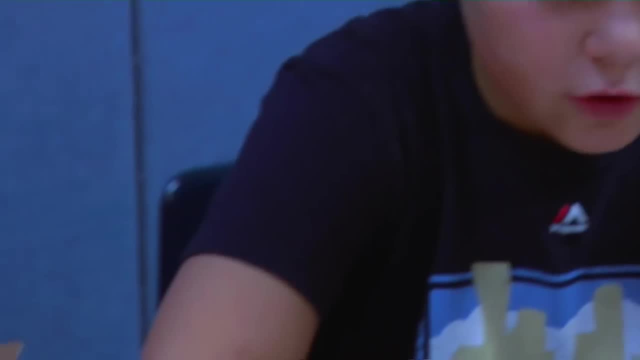 Anna loved her pet dog Buddy. They're going to be reading it together. It might be a repeated reading with comprehension- Anna loved her pet dog Buddy- Where the student will read the same passage multiple times and after each reading, Callie will ask questions. 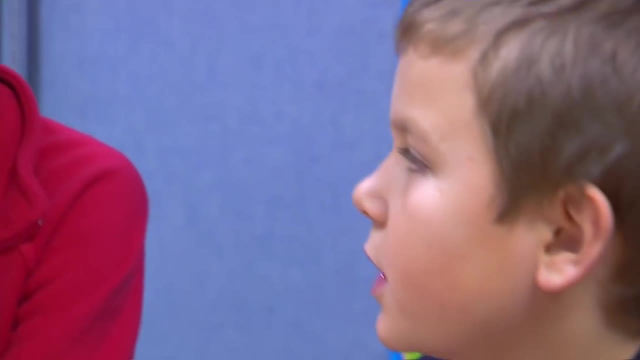 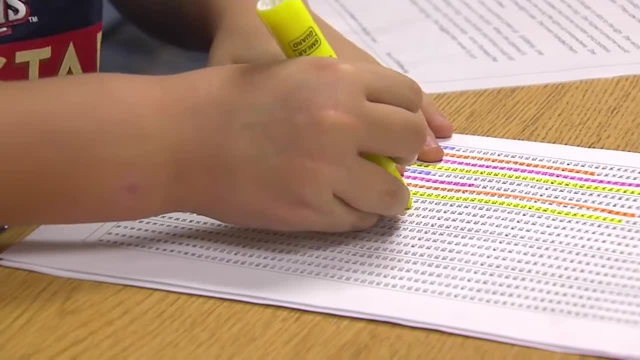 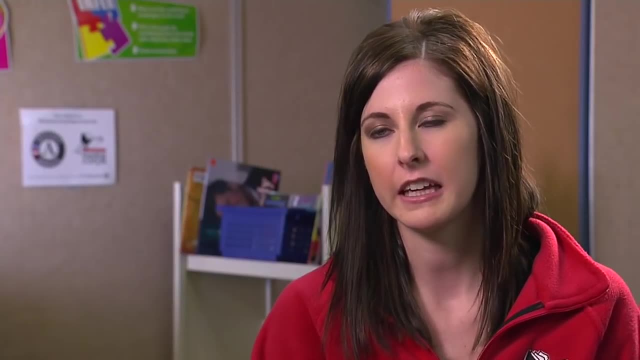 She's going to find Buddy. The student reads the story for one minute and then they actually record how many words they read correct in that minute. so that gives them that sense of accomplishment. and having them graph it and seeing how much they're increasing each time definitely gives them. 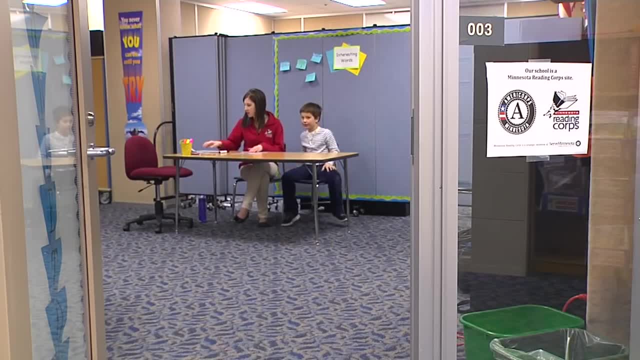 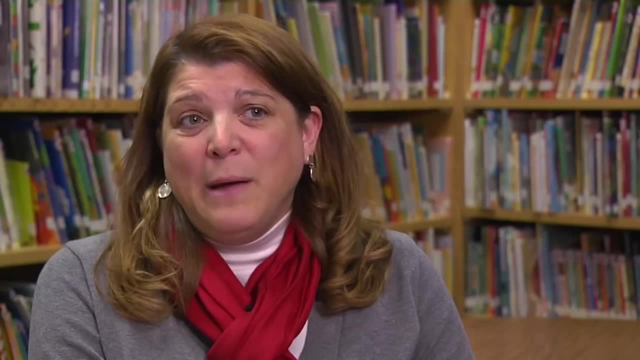 confidence. So great work, Anna. how about that? Awesome? The student is excited because they know in that room, with that Minnesota Reading Corps tutor, they're going to be successful And for some students that may be the only 20 minutes of the whole day that they really feel successful. It builds their confidence. 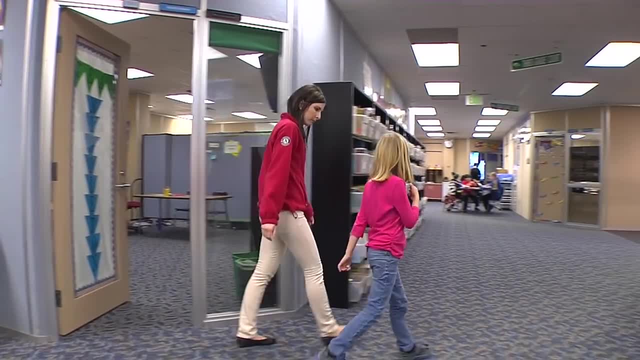 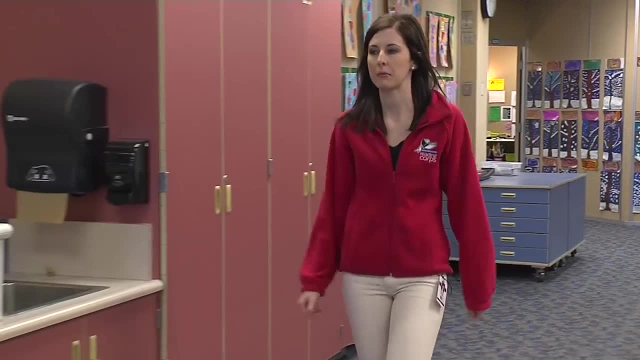 and then they can go back into the classroom, use that confidence they have. So in our building it makes a big difference. It's great to know that I do make a difference. here at the school We have many different people that decide to become a tutor.